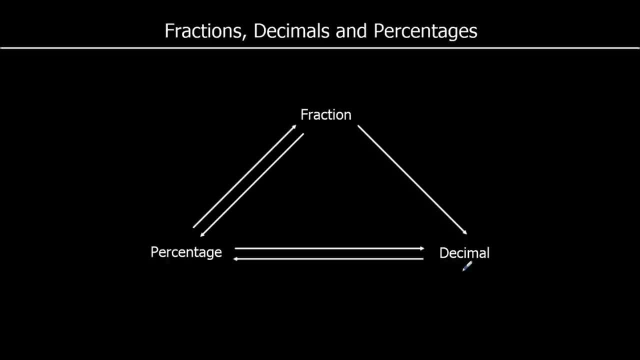 So say, we started with a decimal and we started with 0.3. If I want to change a decimal to a percentage, I multiply by 100. So I can change a decimal to a percentage by timesing by 100. 0.3 times 100, that's the same as timesing by 10 twice. 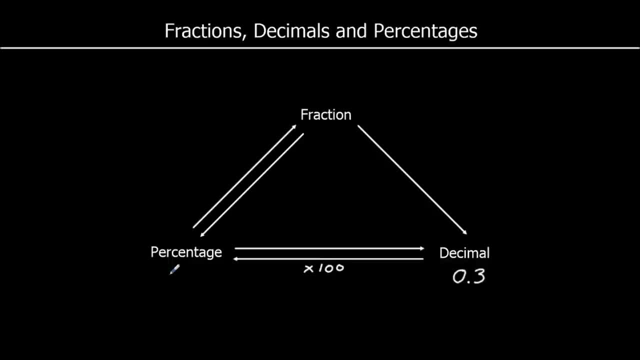 So times 10 once for 3, times 10 twice will be 30. And we write that as 30, with a percent sign 30%. If I wanted to change a percentage back to a decimal, I'll do the opposite, which is dividing by 100. 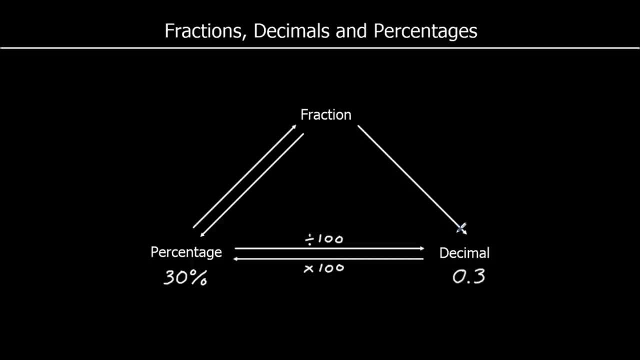 So decimal to percent times 100, percent back to decimal, divide by 100.. To change a percentage to a fraction I can just rewrite the percentage as a fraction. So a percentage is really a fraction out of 100.. So 30% means 30.. 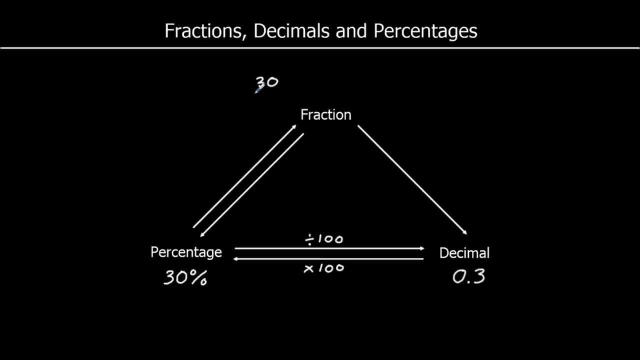 So 30% is really over 100. So if ever you've got a percent, that's the same as a fraction out of 100. And I can simplify this fraction. I can say they're both in the top and bottom, are both in the 10 times table. 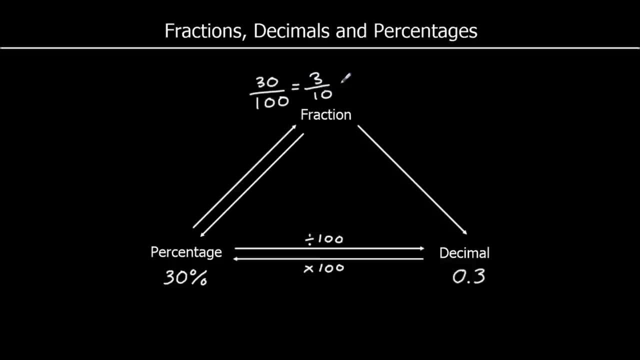 So I've got 3 tenths. So to convert a percentage to a fraction, we can rewrite the percentage. So we can write over 100 and simplify. To change a fraction back to a percentage, we can either do the opposite, which is make the fraction out of 100 and then rewrite it as a percentage. 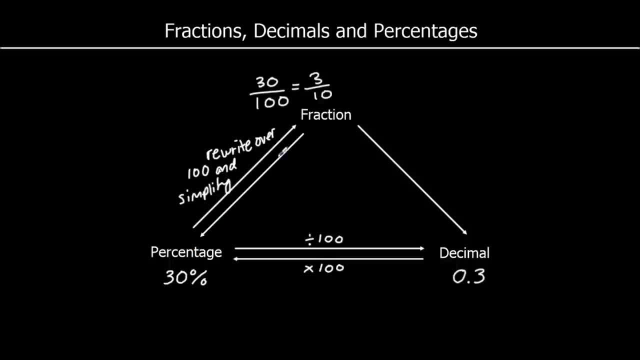 Or we can times by 100.. So either times by 100, or write over 100.. To change a fraction to a decimal, we take the top number and divide by the bottom number, So 3 divided by 10 in this case. 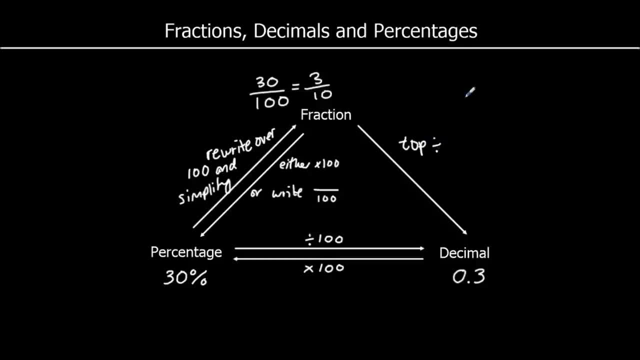 So top divided by bottom, or you could say numerator divided by denominator. So 3 divided by 10 is 0.. So 3 divided by 10 is 0.. So I'm going to go over each of these in a bit more detail now. 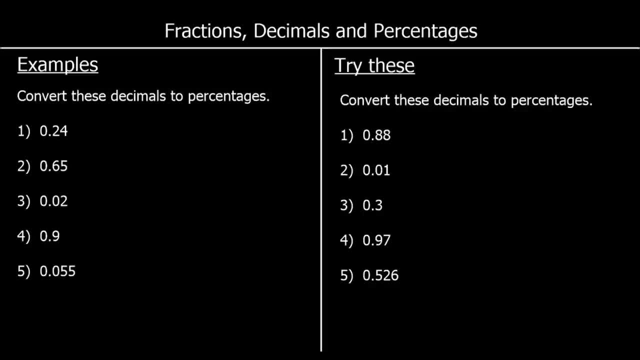 So these first questions are converting decimals to percentages. To convert a decimal to a percentage, we're multiplying by 100. So we're going to multiply each of these by 100. So 0.24 times 100 times 10. once is 2.4 times 10, twice is 24.. 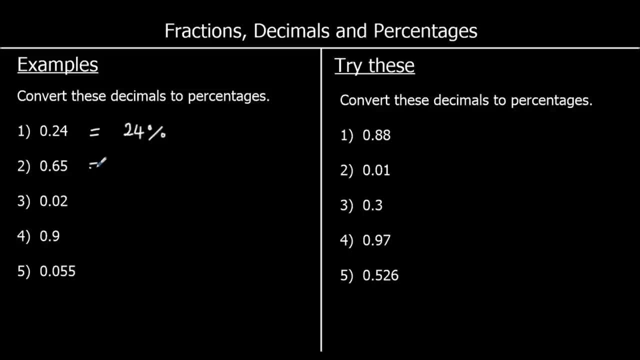 So it's 10 times 2.4.. So it's 24% 0.65 times 100, 65% 0.02 times 100, so times 10 once will be 0.2.. Times 10 twice will be 2.. 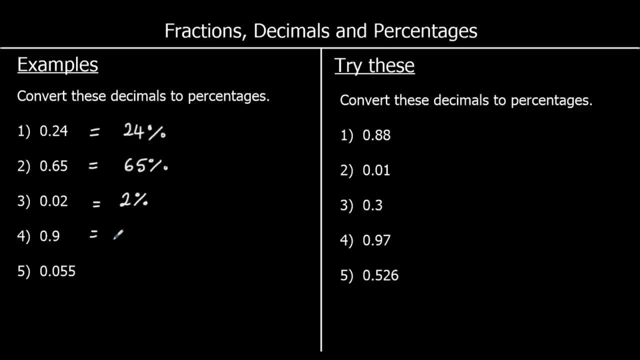 0.9,. so times 10 once for 9, times 10 twice is 90.. And 0.055 times 10 once is 0.55.. Times 10 twice and that'll be 5.5.. 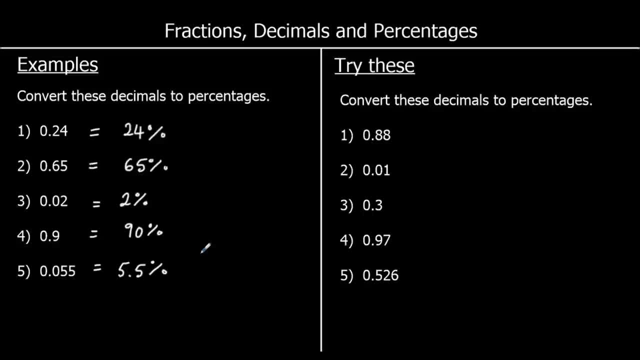 So it's 5.5%. 5 for you to try here. give them a go. Question 1, we've got 0.88.. So that is 88%. 0.01 is 1%, 0.3 is 30%. 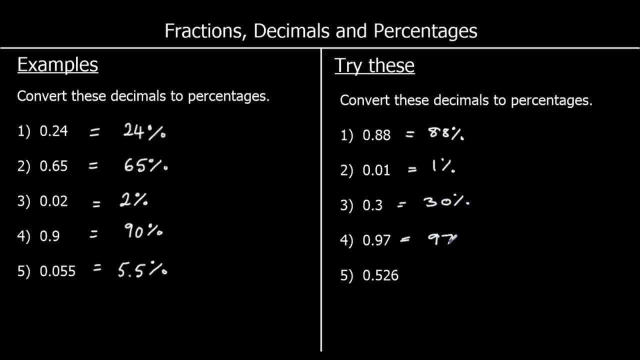 0.97 is 97% And 0.526 is 52.6%. So each time we're multiplying by 100.. To convert from a percentage to a decimal, we're going to do the opposite, So we are going to divide by 100. 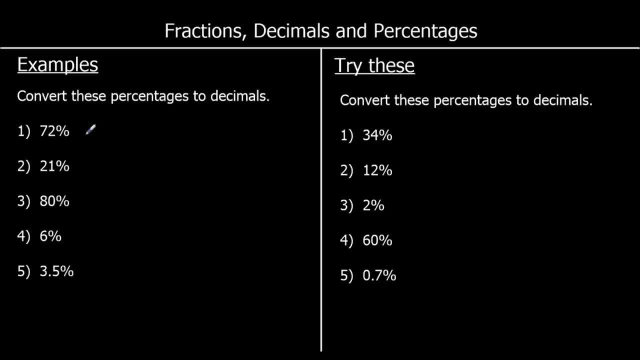 So 72% divided by 100.. Divide by 10 once be 7.2.. Divide by 10 twice 0.72.. 21%. So 21 divided by 100 is 0.21.. 80 divided by 100.. 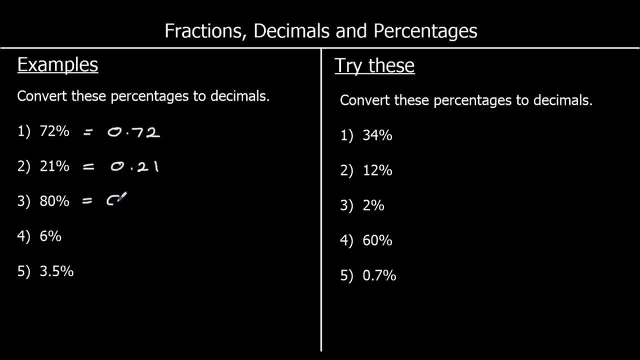 Divide by 10 once is 8.. Divide by 10 twice is 0.8.. 6 divided by 100.. So 0.6, and then 0.06.. And 3.5 divided by 100.. So divide by 10 twice. 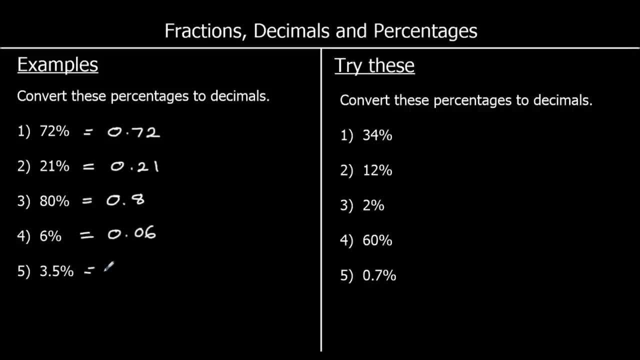 We've got 0.35, and then 0.035.. So 5 for you to try Convert the percentages to decimals. So each time divide by 100.. Question 1, you should have 0.34.. Question 2,: 0.12.. 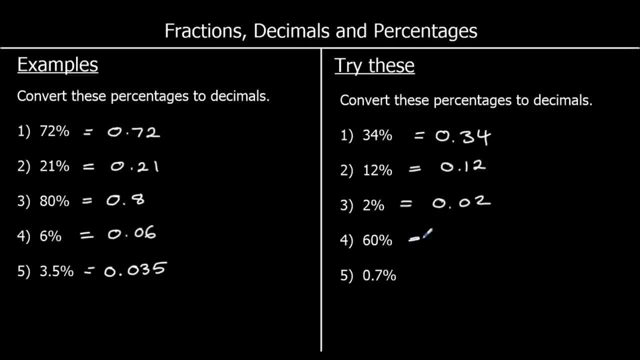 The 2% is 0.02.. 60% is 0.6.. And 0.7% is 0.6.. 0.6 is 0.6.. 0.6 is 0.6.. 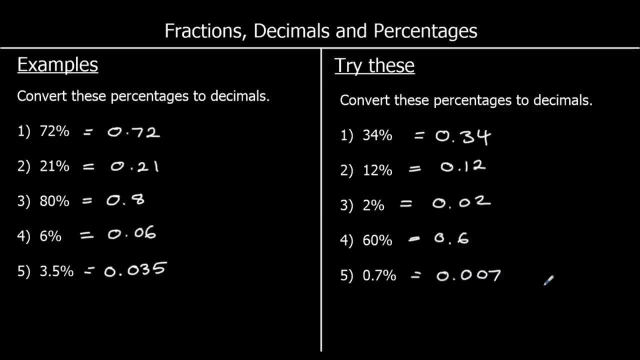 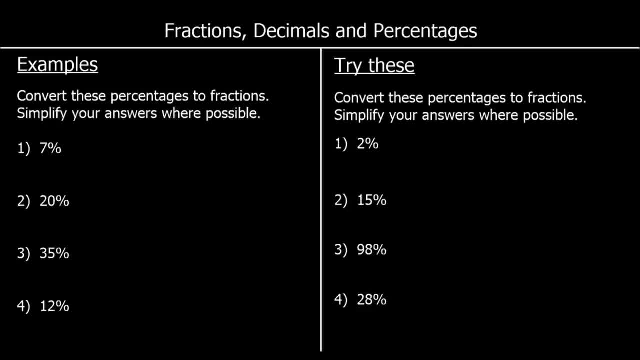 Convert these percentages to fractions. So remember, percent means out of 100.. So percent out of 100. So we can read: write a percentage as a fraction out of a hundred, and we're going to simplify answers if we can. so seven percent means seven hundredths, seven out of a hundred. 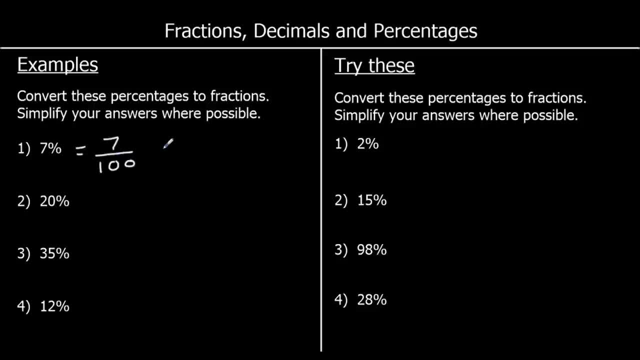 seven and a hundred. well, seven is a prime number. seven and a hundred aren't in the same times table, so that is as simple as it gets. twenty percent means twenty over a hundred, twenty and a hundred to both in the- well, the biggest times table is a. 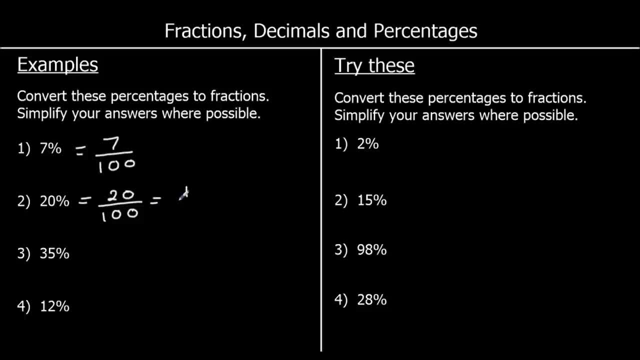 twenty times table. so it's one twenty and five twenties 35%, so thirty five over a hundred, and they are both in the five times table. so we've got seven. fives makes thirty five, and twenty fives Make 100 and 12 percent, so 12 over 100.. 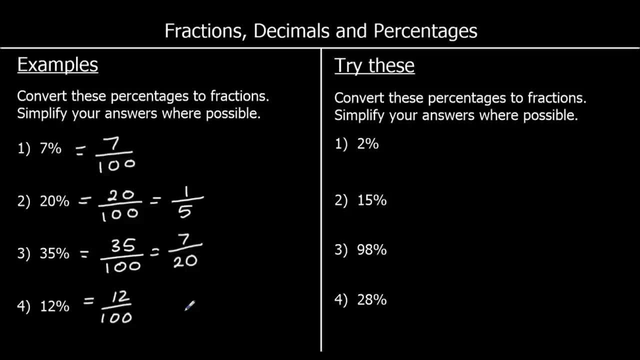 And we can say they're both in the four times table. So we've got three twenty-fifths. You could have halved it and halved it again. You should get the same answer. Okay, four for you to try, so give them a go. 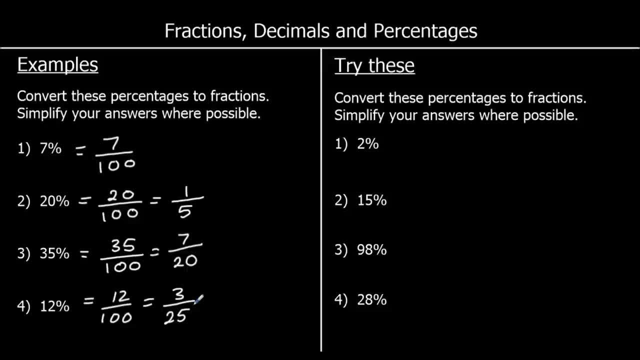 Okay, question one: we've got two percent, so that's the same as two over 100.. They're both even, so we can half them. so one fiftieth Fifteen percent is 15 over 100. And they are both in the five times table, so it's three twentieths. 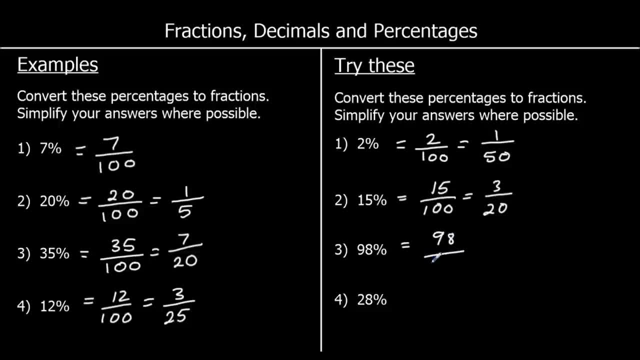 Ninety-eight percent is 98 over 100. And they're both, even so we can half them. both Forty-nine over 50. And twenty-eight percent is 28 over 100. And we can do it in steps if you want. 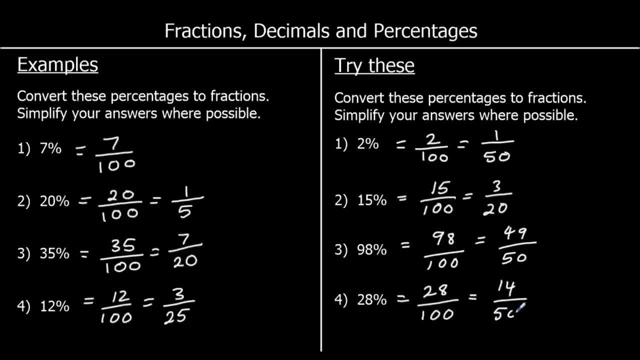 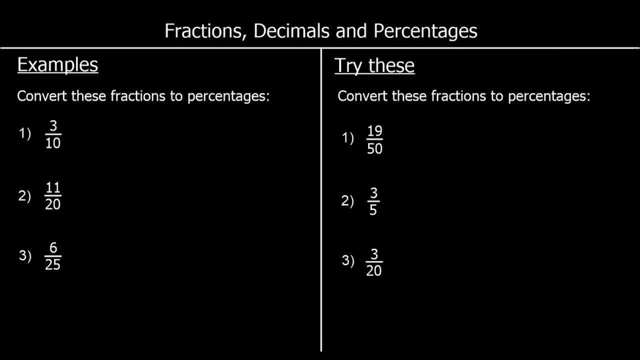 We can half them both, so 14 over 50.. And then half again, seven over 25.. You could have divided it by four to start with, But either way you get the same answer. Convert these fractions to percentages. So we can convert fractions to percentages by doing the opposite. 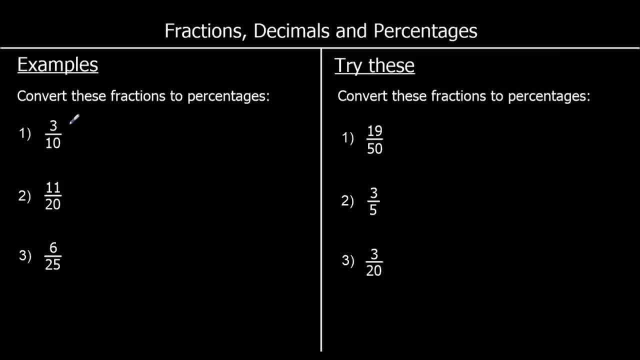 which is making the fraction out of 100.. So how can we make three tenths out of 100?? If we times top and bottom by the same thing, the fraction stays equivalent. So we can change a fraction by times including Top and bottom by the same thing. 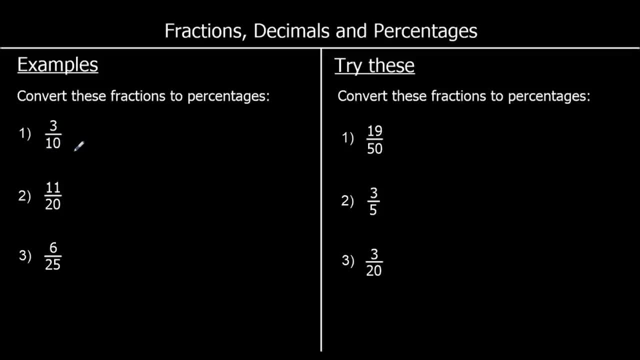 So to make the bottom, the denominator 100, we need to times by 10. So we'll times the numerator, the top number, by 10 as well. So that makes 30 out of 100.. And 30 out of 100 is 30 percent. 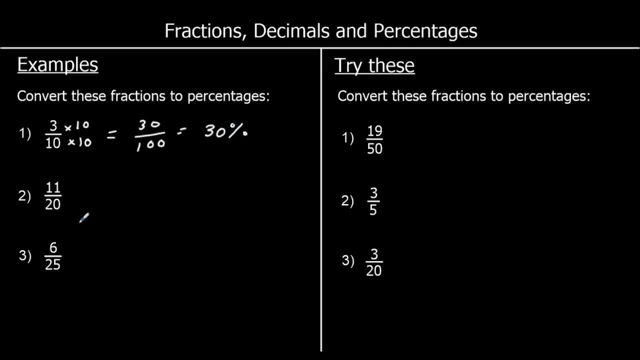 Eleven, twentieths. for question two, To make our bottom number, our denominator, our denominator, 100, we're going to multiply by five, And whatever we multiply the bottom by, we need to multiply the top by the same thing. So that gives us 55 out of 100. 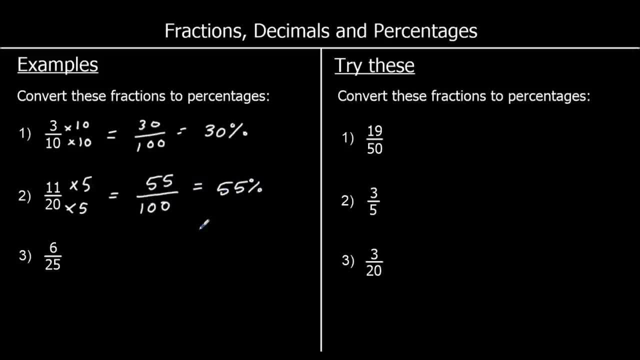 Which is 55 percent, And the third one to make our denominator 100, we're going to multiply by four, So we're going to multiply top and bottom by four, Six, fours, So twenty four. Twenty four over 100 is 24 percent. 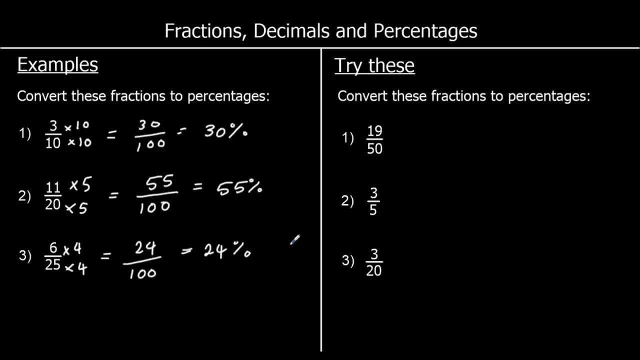 OK, three for you to try, So give them a go. Question one: let's multiply top and bottom by two, So we've got 38 out of 100, which is 38 percent. Question two: We're going to multiply top and bottom by 20, so we've got 60 out of 100, or 60 percent. 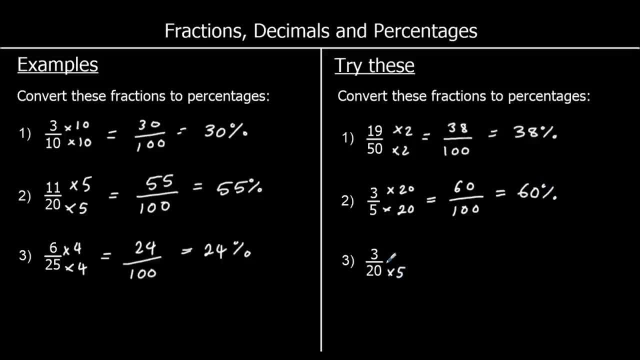 And question three: multiply top and bottom by five, So we've got 15 out of 100, or 15 percent. And the last one: we're going to convert fractions to decimals. So to convert a fraction to a decimal, we're going to divide the top number by the bottom number. 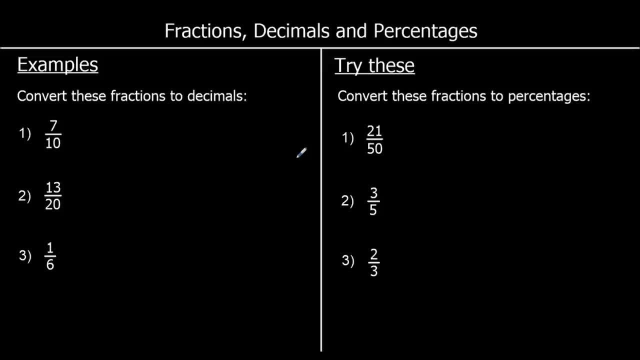 We can always rewrite a fraction as a division. So if you look at the divide sign, it looks like a fraction And it's seven divided by 10.. Seven tenths is the same as seven divided by 10.. So if we do seven divided by 10.. 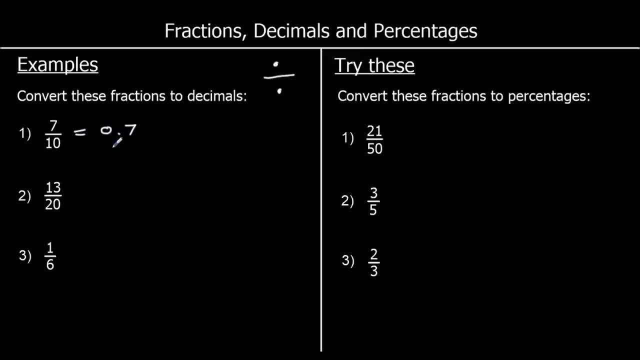 We get 0.7.. And that is a decimal For question two. we've got 13 divided by 20.. And that looks complicated. But what we can do is we can make it out of 100 or make it out of 10 to make our division easier. 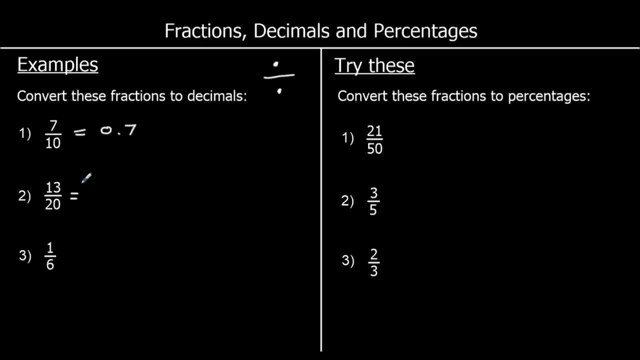 So if we even multiply top and bottom by five to make it out of 100, which we'll do So- 13 times Five is 65.. 20 times five is 100.. So it's 65 over 100.. And 65 divided by 100 is 0.65. 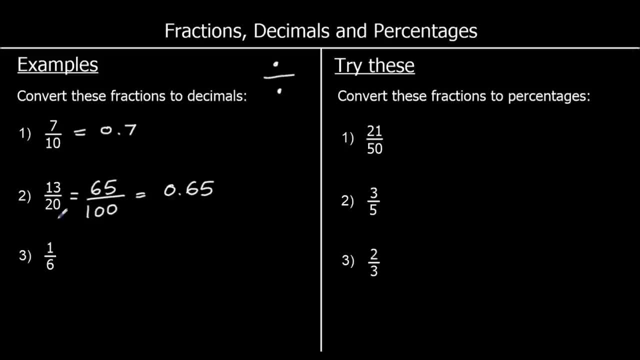 We could have also half top and bottom and had 6.5 over 10.. And 6.5 divided by 10 is also 0.65.. And the third part, one, one, six. now, this one is a lot harder, so we need to do one divided by six. but 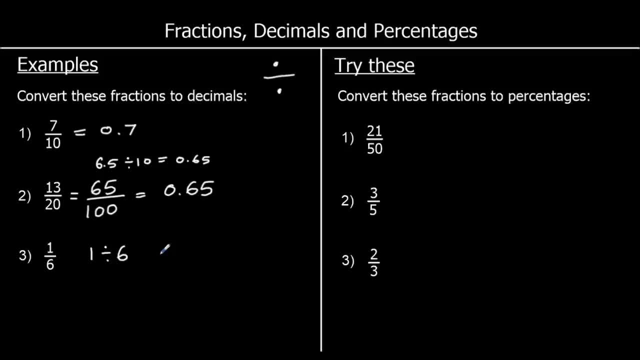 there's no way of making this an easy calculation, so we are gonna have to use our short division method. so how many sixes go into one? so that's right. one point: zero, zero, zero, zero. so how many sixes are going to go into one? it's. 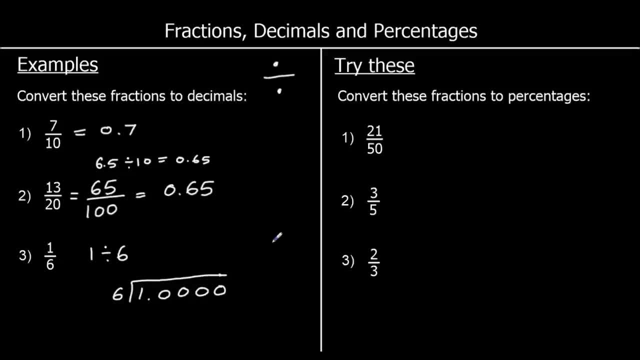 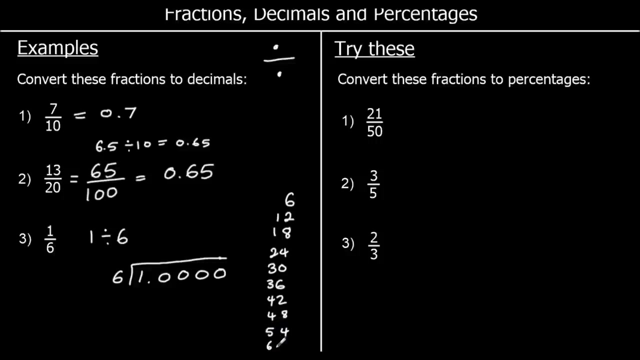 gonna be a decimal, so I've added all these zeros. I'm gonna write the six times table down the side. so six, twelve, eighteen, twenty four, thirty, that's five sixes. thirty six is six squared, and forty two, forty eight, fifty four and sixty, so all the way up to ten. so how many sixes go into one? that's zero. 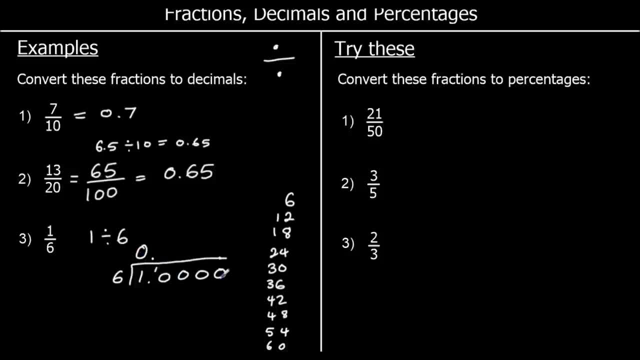 and we've got one to carry over. one left over. how many? six is going to ten? that's one. with four left over. how many? six is going to forty? that's six, six, six is a thirty six and we've got four left over. how many? six is going to forty at. 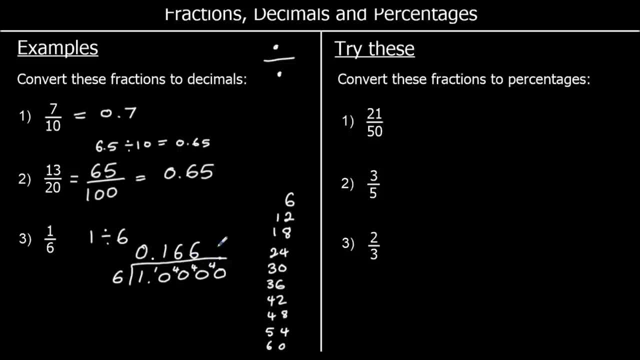 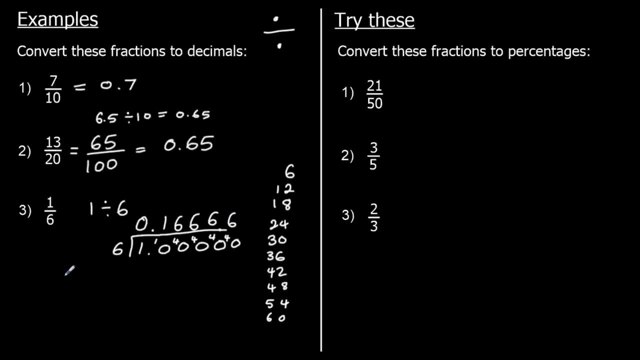 six with four left over, how many six is going to forty? that's six with four left over, and so on. so one six as a decimal is zero point one, six, six, six, six, going on forever. so we can write that zero point one, six recurring if we 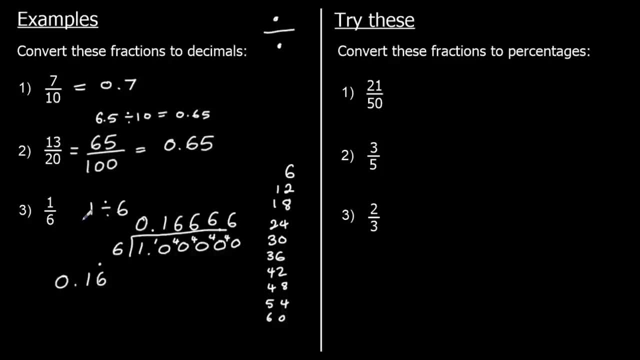 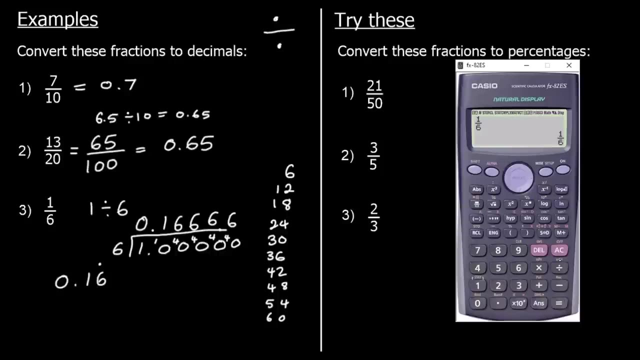 had a calculator, this would have been a lot easier. we would have just written one divided by six, or even one sixth, into the calculator and it would have given us the answer. so if we wrote one sixth into the calculator and press the s2d button, it would tell us it's zero point one, six. recurring zero point one, six, six, six, six. 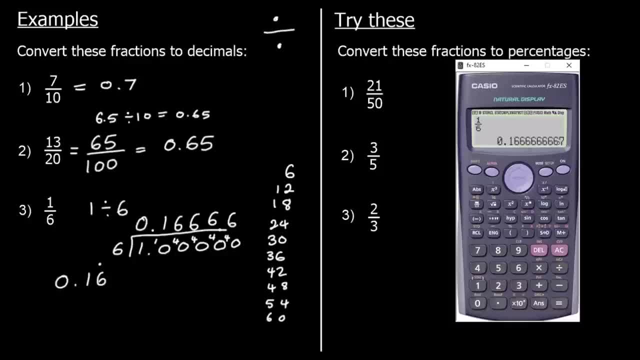 six, six, six, going on forever. the calculators put a seven on the end because the calculator is rounded. we can do any fraction, decimal and percentage version in the calculator. if you start with a percentage, so 26%, use the percent button on the calculator, press equals. it's going to change it to a fraction straight away for you. And if you 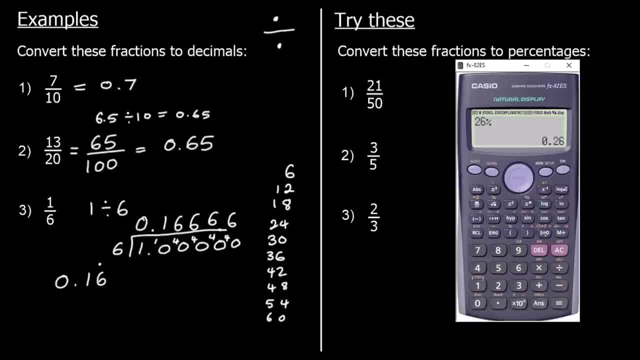 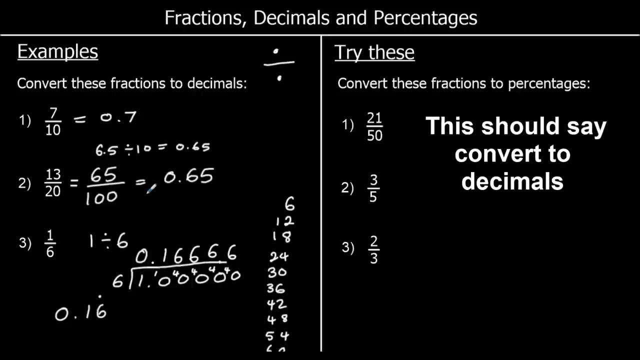 press the S to D button, you're going to get a decimal as well, And if you started with a decimal, the calculator will turn it into the fraction for you. Okay, three of these for you to try. So 21 over 50 doesn't look easy, But if we double the top, 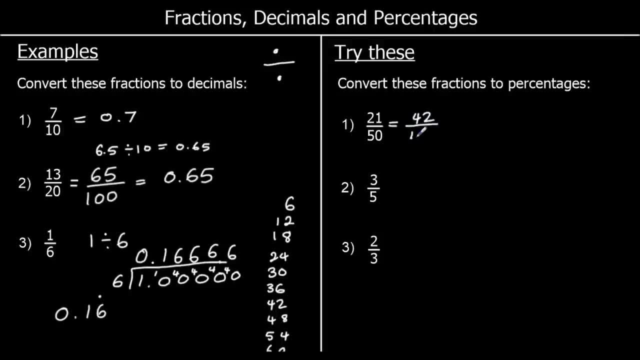 and the bottom. so it's 42 out of 100.. That's a lot easier to divide. So 42 divided by 100 is 0.42.. For three fifths, again, three divided by 100 is 0.42.. So that's a lot easier to divide. 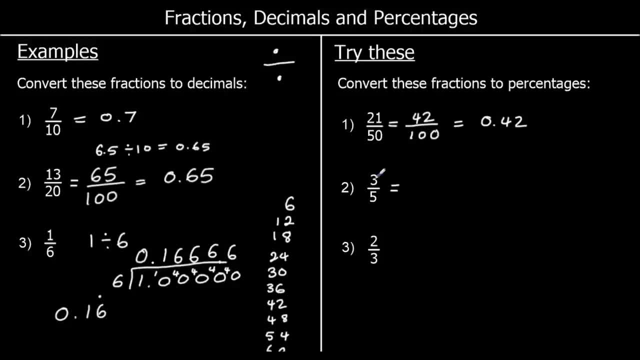 Divided by five isn't very easy, But we can change the calculation, double top and bottom And we'll have six divided by 10, which is 0.6.. And two thirds. if you already know what two thirds is as a decimal, you can just write down the answer. It's one that people might remember. 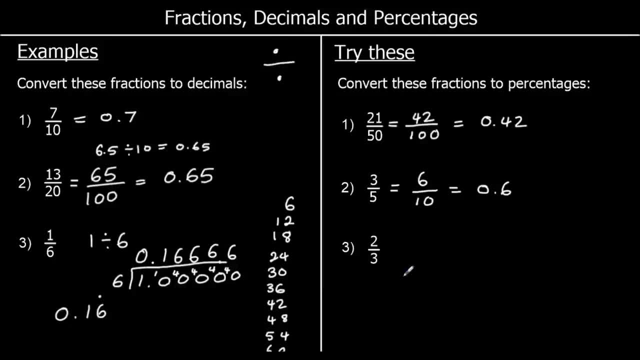 Or the alternative is to see how many threes go into two. Three is going to two, point. We'll add some zeros, 2.0000.. Write down the three times table: How many threes go into two. That's zero, Two left over. 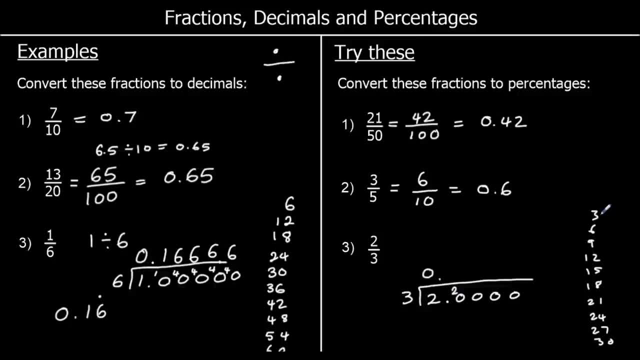 How many threes go into 20? That's six. Six make 18.. With two left over, how many threes go into 20? That's six, With two left over. how many threes go into 20? That's six, with two left over, and so on. 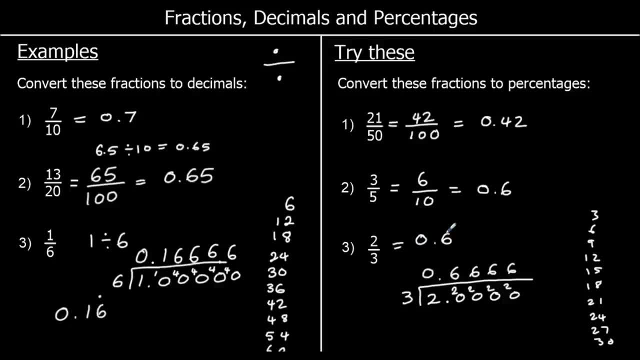 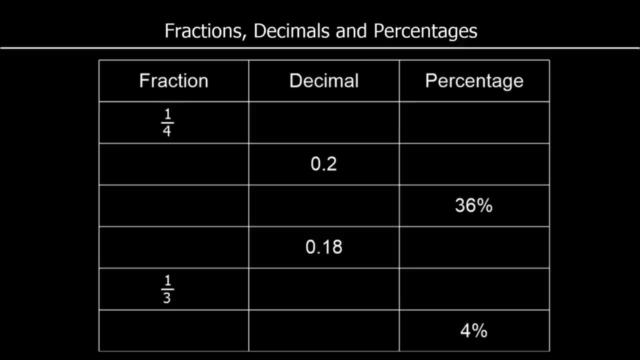 So two thirds is 0.6, recurring 0.6, going on forever: 0.66666666.. So that was converting between fractions, decimals and percentages. To finish up, we've got a table here converting between fractions, decimals and percentages and see if you can fill in the gaps. 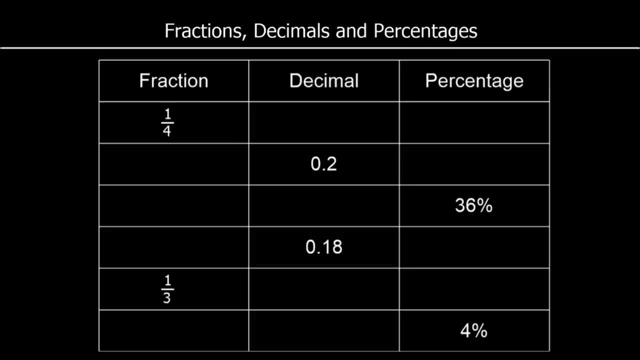 The first one is one quarter. so we've got one quarter, which is a fraction, and we need to write that as a decimal and a percentage. This might be one of the ones that you know, and that is 0.25 as a decimal and 25%. 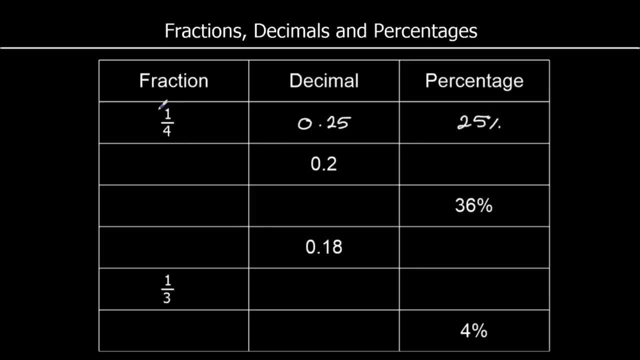 You could have done 1 divided by 4 to figure it out if you didn't know it. For the second one, we've got 0.2, which is a decimal. To convert it to a percentage, we can times by 100. 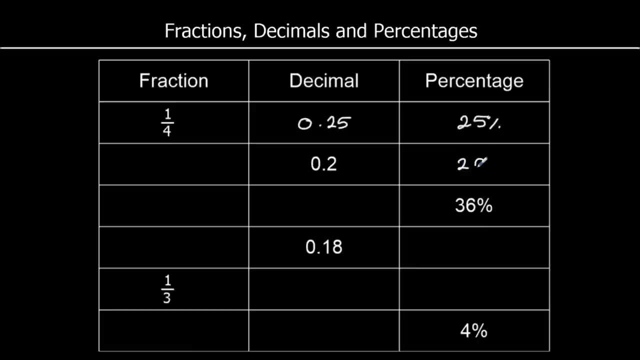 So times by 10 twice, which is 20%, And then to write that as a fraction that's 20 over 100.. But they're both in the 20 times table, so it simplifies to one fifth: 36% as a fraction is 36 over 100.. 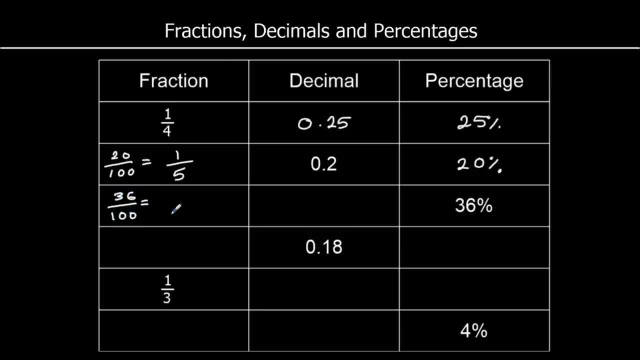 And they're both in the 4 times table. So that simplifies to 9, twenty-fifths, And as a decimal, 36 divided by 100 is 0.36.. 0.18 as a percentage times by 100, so 18%. 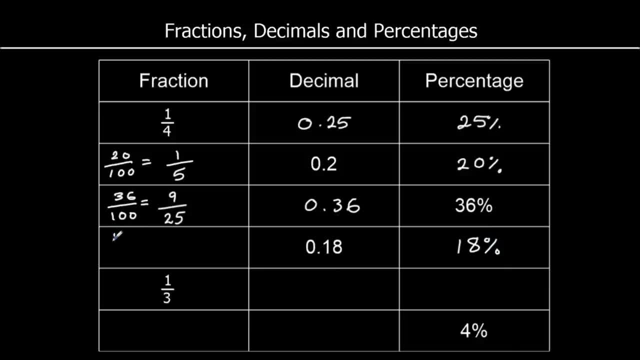 And then we'll write that as a fraction is 18 over 100.. Or 0.18.. We can half top and bottom. 9 fiftieths, One third. hopefully, that's one, you know It's 0.3333. going on forever. 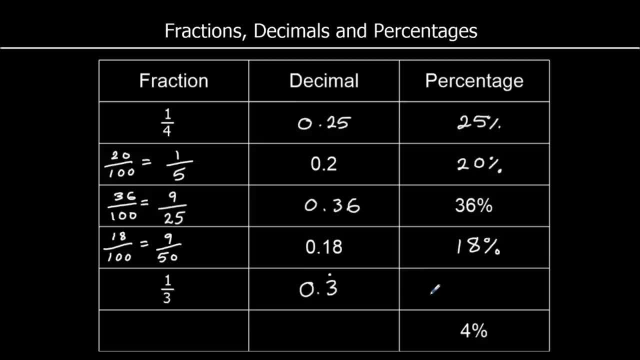 0.3 recurring as a percentage. So 0.3 going on forever times 100 is 33.3 going on forever percent And we've got 4%. So it's a fraction: 4, one hundredths. divide top and bottom by 4 is 1- twenty-fifth. 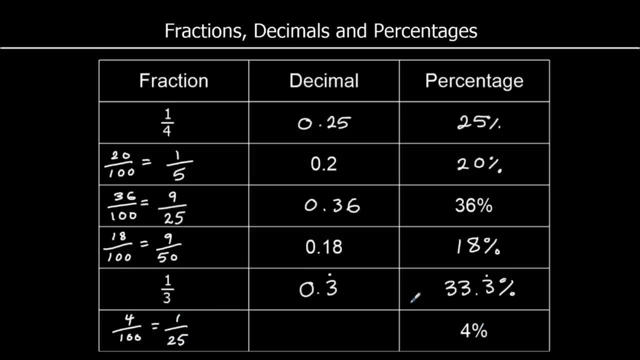 Or as a decimal 4 divided by 100 is 0.04..